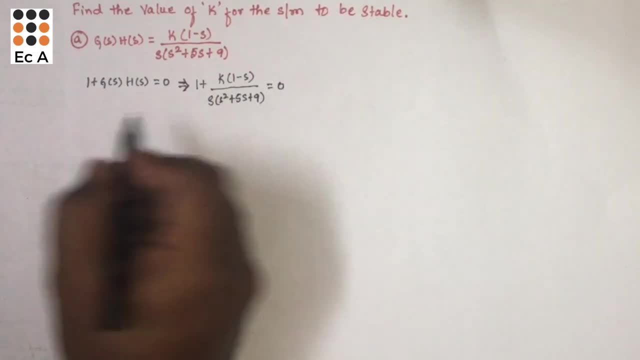 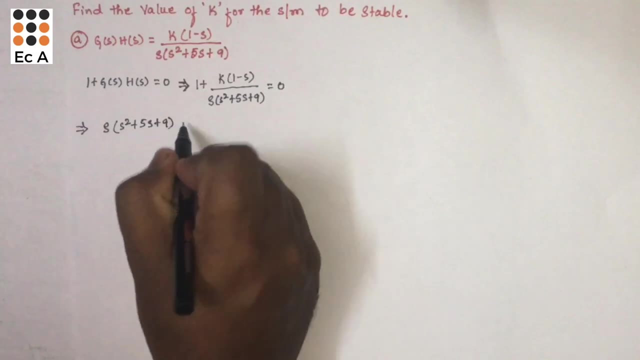 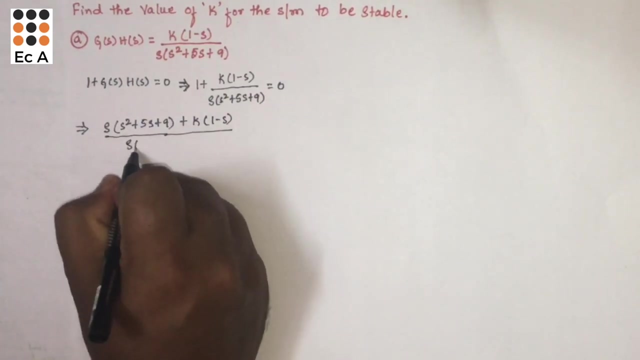 Now in this equation, let us take LCM. We will get s into s square plus 5s plus 9 plus k into 1 minus s. divided by s into s square plus 5s plus 9 is equal to 0.. 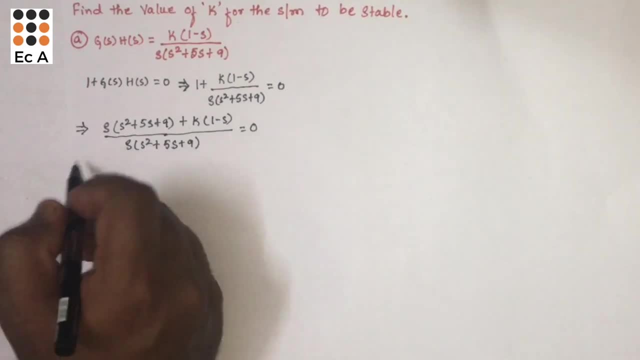 Now we can multiply this denominator with 0.. So we can write the above equation as 1 plus k into 1 minus s. divided by s into h of s is equal to 0.. We can multiply s with this, So it will be s cube plus 5s square plus 9s plus. 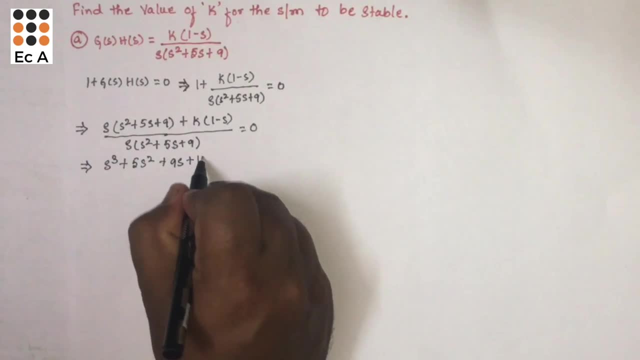 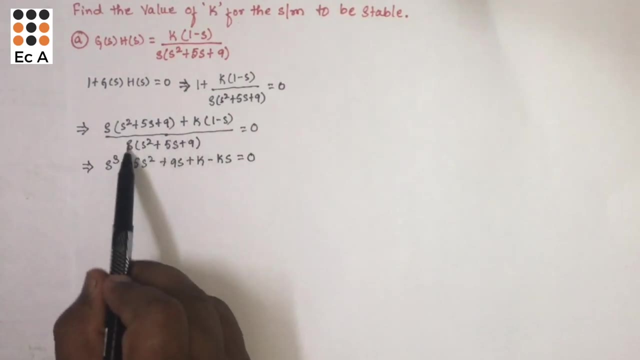 if we multiply k with this, it will be: k minus ks is equal to 0.. So what we have done, We have multiplied this denominator with 0 and we will be left out, with only the numerator. In the numerator. we have simplified the equation. 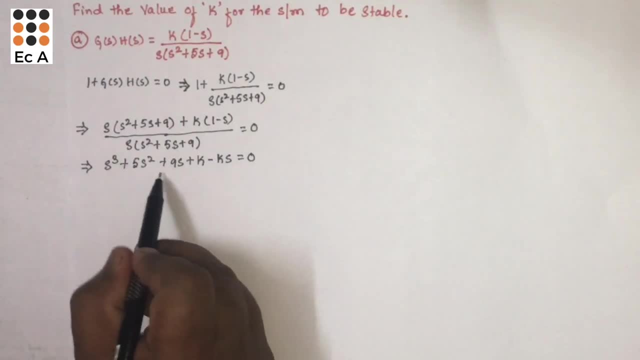 And whatever equation we have, we have to write the denominator with 0. So what we have got here, it is the characteristics equation. So from this characteristics equation we need to find the range of k for which the system is stable. 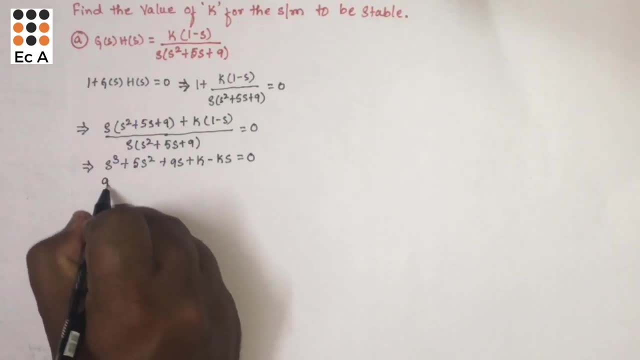 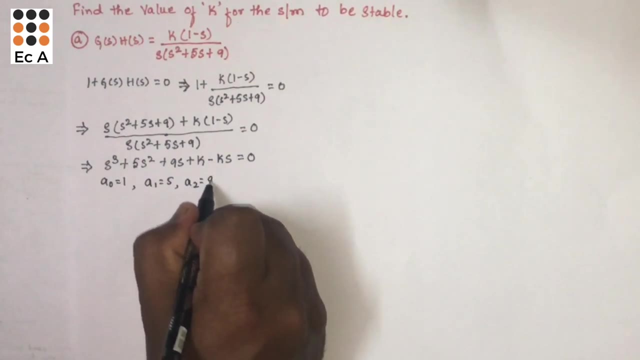 So from this characteristics equation we can write: a0 is equal to 1, a1 is equal to 5, a2 is equal to 9 minus k and a3 is equal to k. So this is the s cube term. 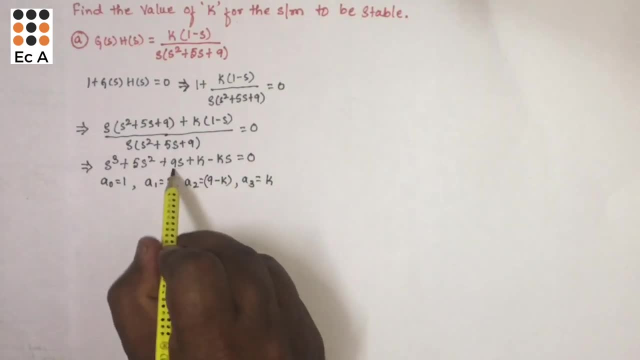 This is s square term For s. we can write it as 9 minus k, So that's why we have written a2 as 9 minus k. Now let us write the Roth's table. So the highest power of s is s cube. 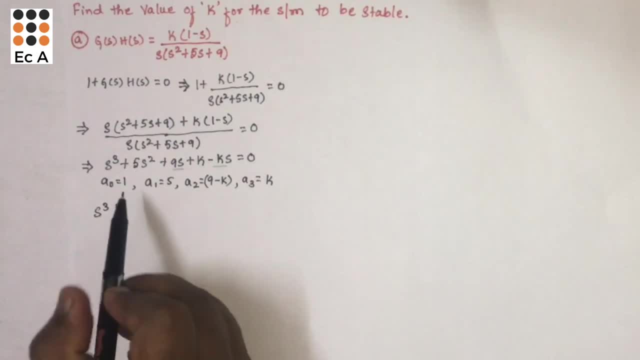 Let us take s cube. In the first row we will write a0, a2.. So a0 is 1, a2 is 9 minus k. Let us take s square. In the second row we will write a1, a3.. 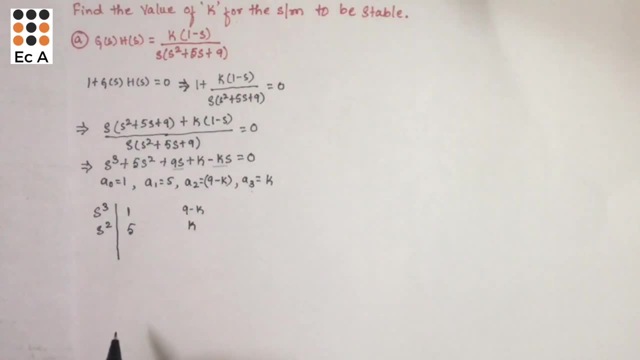 So it will be 5 and k. Now we need to find the row s to the power of 1.. So for that we need to multiply 5 into 9 minus k minus 1 into k divided by 5.. 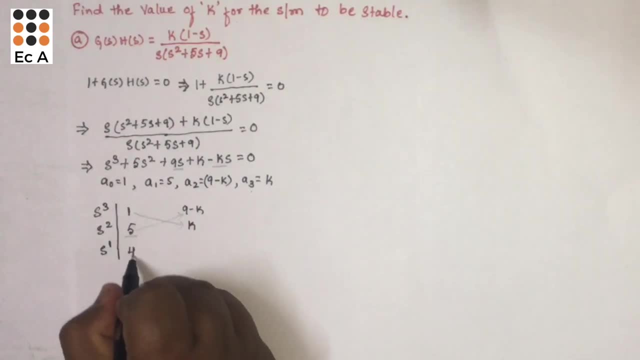 So we will get 45 minus 5k minus k divided by 5.. And next term we don't have, We can take it as 0.. Now let us find s0.. To find s0, this entire term is multiplied with k minus 5 into 0, divided by this term. 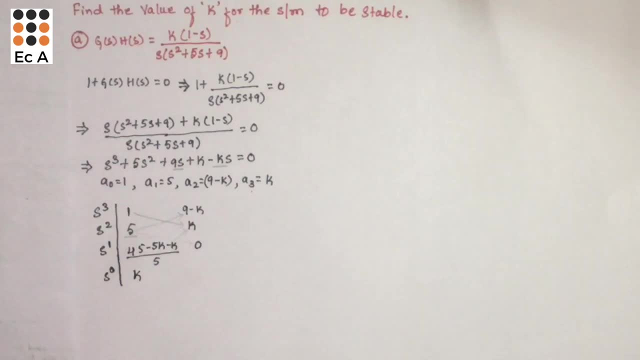 So we will get s to the power of 0 as k. So after writing the Roth's table, from this table we can write from the row s0, we can take the term k And we can say: this value should be greater than 0, so that the system should be stable. 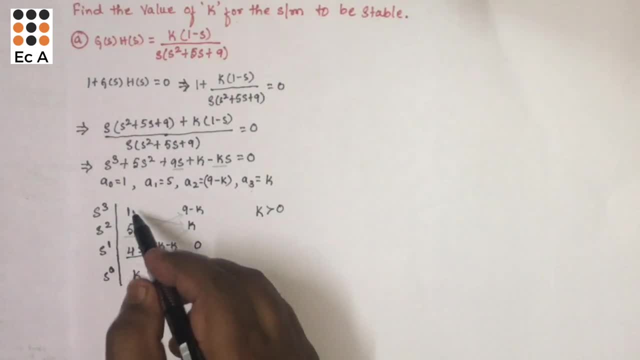 We know the condition for stability. For stability, the first coefficients in the column should be positive, so that the system should be stable. So positive, which means it should be greater than 0.. So that's why, from the row s0, we have taken k. 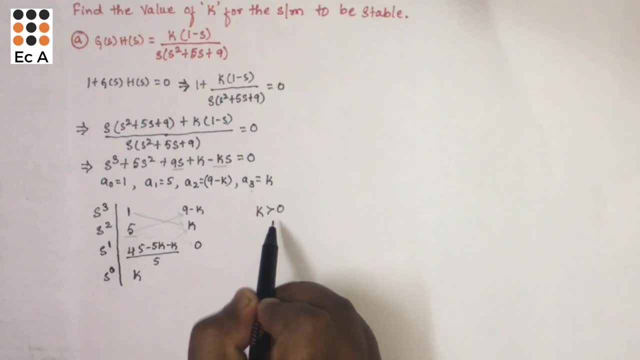 And we know the condition is k should be greater than 0. And this is one condition. And from the row s to the power of 0, the power of 1, we can write 45 minus 6k. we have written minus 5k minus k, as 6k divided by 5. 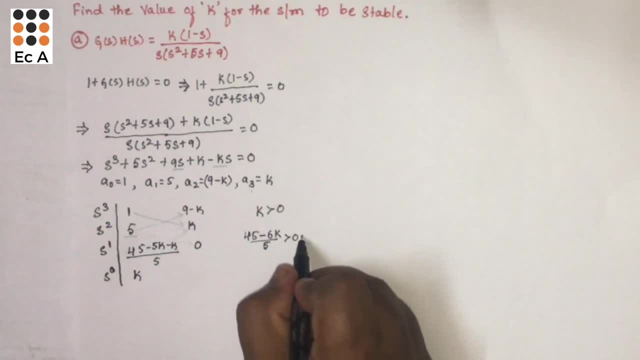 should be greater than 0. so from this we can write: 45 minus 6k should be greater than 0. from this equation we can write: 45 should be greater than 6k. or we can write k should be less than 45 divided by 6, so we get k should be less than 7.5, so we got two ranges of k. 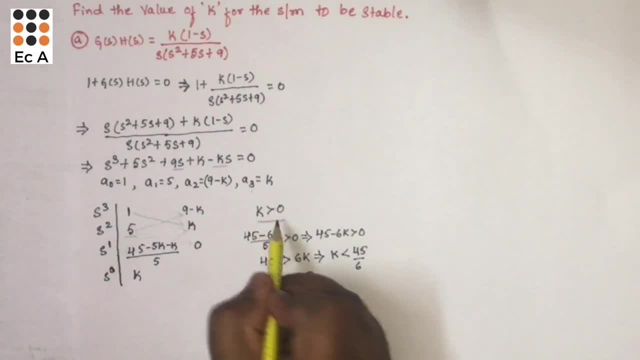 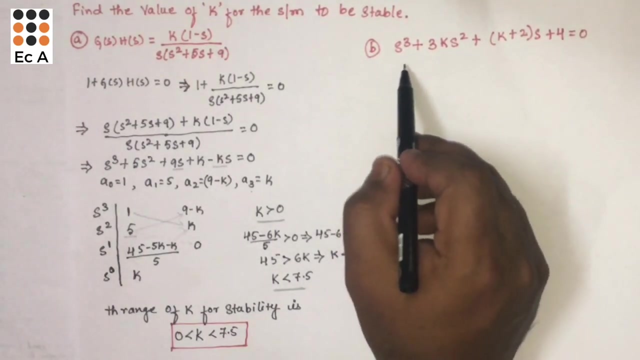 so which is k should be greater than 0 and k should be less than 7.5. so we can say the range of k for stability is k should be greater than 0 and less than 7.5. let us take the second problem. here they have given the characteristics equation directly. 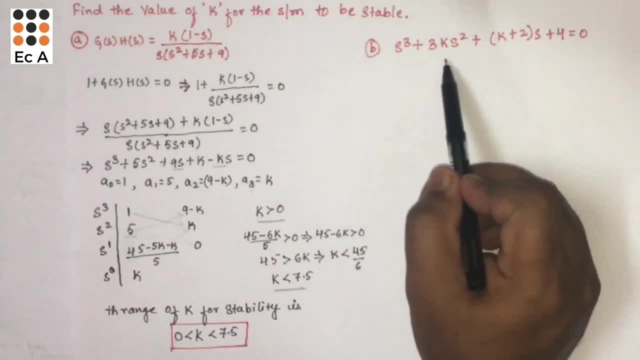 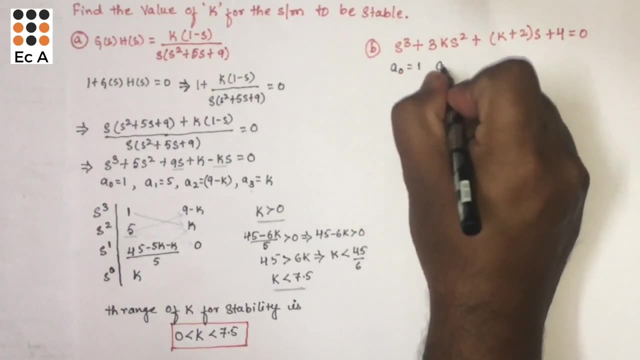 so instead of giving g of s into h of s, the characteristics equation is given directly here. so from this characteristics equation we can write: a naught is equal to 1, a1 is equal to 0 and k is greater than 0. so from this we can write: k should be less than 0. 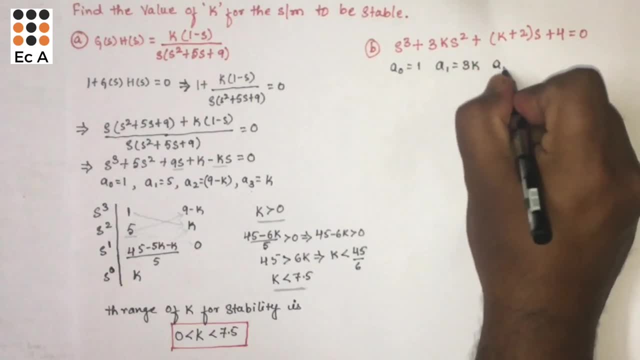 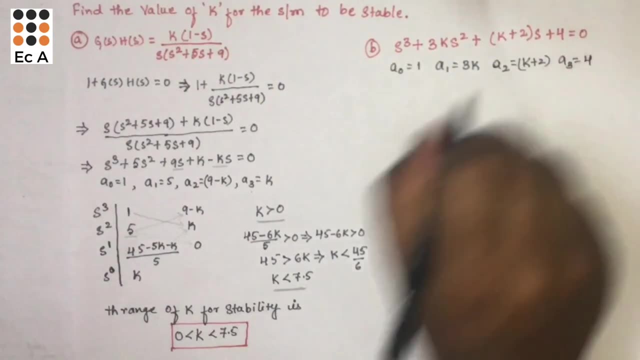 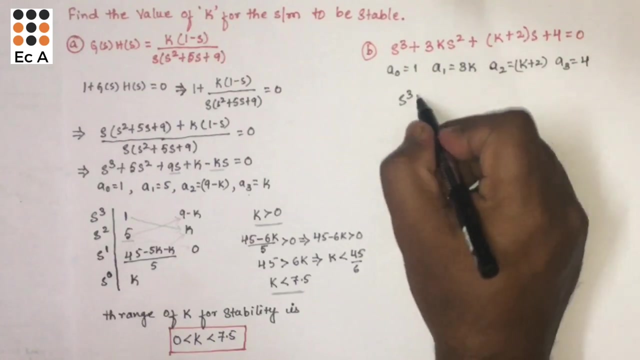 to 3k, a2 is equal to k plus 2 and a3 is equal to 4.. Now let us write the Roth's table. So the highest power of s is cube s cube. In the first row we will write a0,. 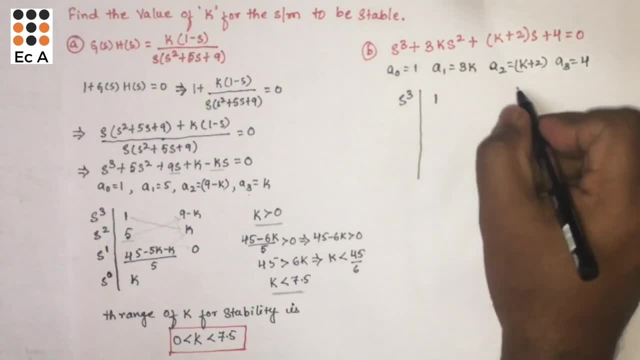 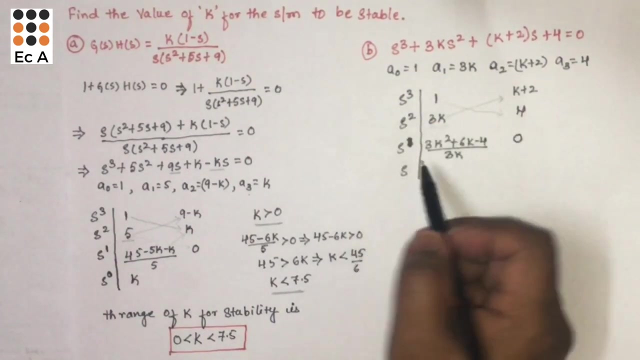 a2, so it is 1 and k plus 2.. In the second row, we will take s square. we will write a1 and a3, it will be 3k and 4.. So we need to find the row s to the power of 1. To find: 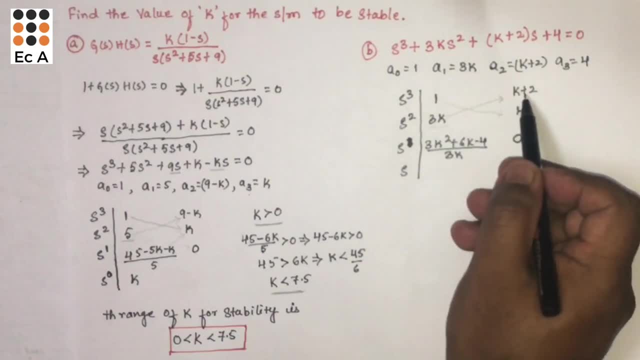 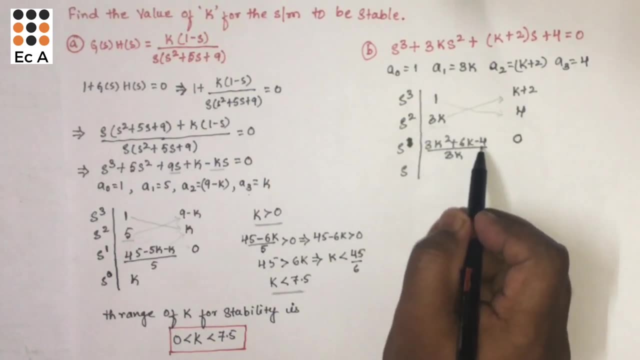 s to the power of 1, we need to multiply 3k into k, plus 2 minus 1 into 4 divided by 3k. So it will be 3k square plus 6k minus 4 divided by 3k. The next term we do not have, so we can. 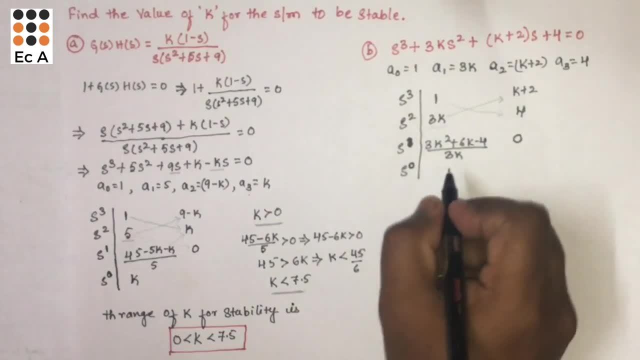 write it as 0.. Next we will find s to the power of 0.. To find s to the power of 0, we will multiply s to the power of 0. So we will write s to the power of 0.. So we will. 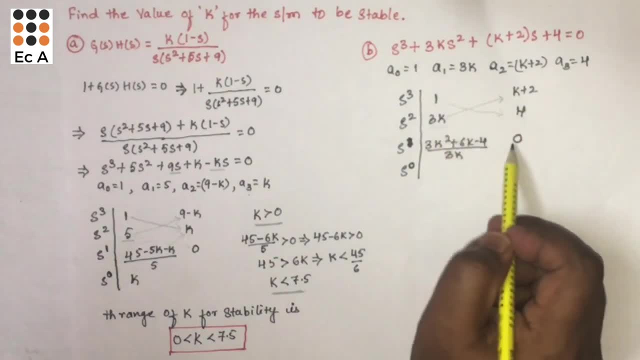 multiply this entire term with 4 minus 3k into 0, divided by this term, So we will get 4.. Now we need to consider the first column. If we take the row s square, from there we can write: 3k should be greater than 0 for the system to be stable. From this we can: 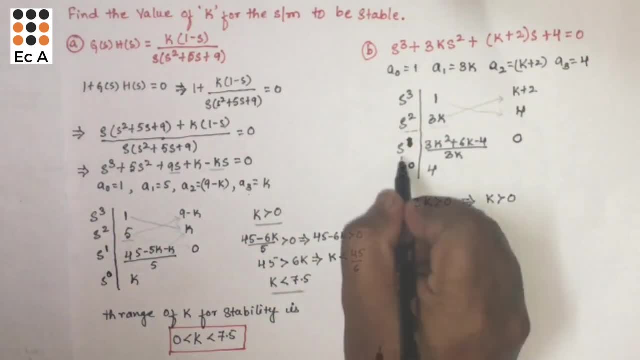 write k is greater than 0. We can take the row s to the power of 1 and we can write 3k square plus 6k minus 4, divided by 3k should be greater than 0. From this we can write: 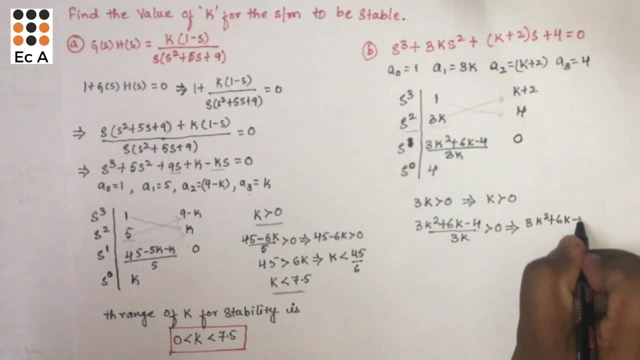 3k square plus 6k minus 4 should be greater than 0.. So from this we will get the roots of k. So we will get k should be greater than 0.5275 and we will get one more root, which is k should be. 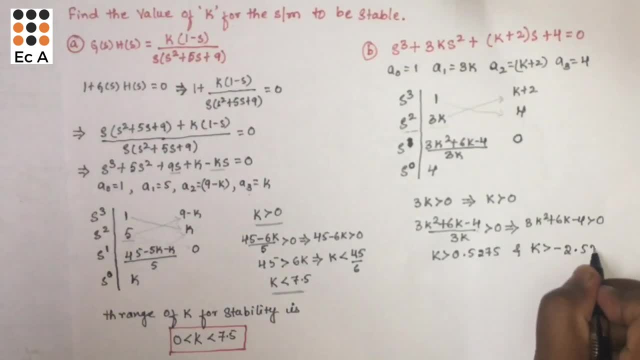 greater than minus 2.5275.. So here we got three values for k, which is: k is greater than 0, k should be greater than 0.5275 and k should be greater than minus 0.5275.. So in these three,